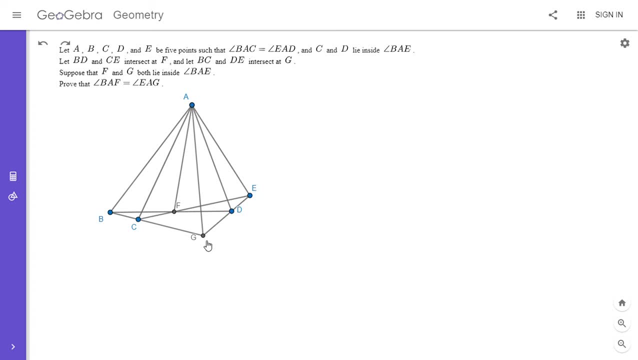 is equal to E A B. Let B C intersect D, E at G. Let B C intersect D E at G, equal to angle EAG. So when I first solved this problem, my solution was a little messier, using. 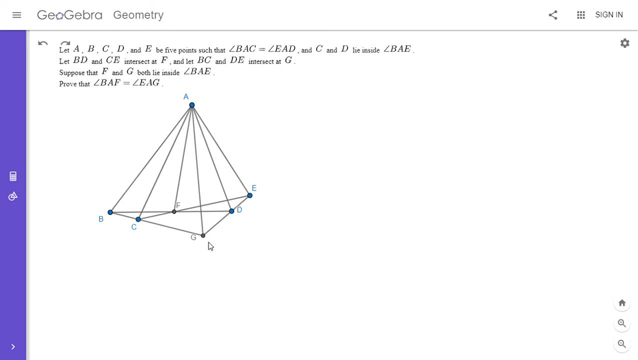 trigonometry. but then I found a really nice solution by the poster, Jean-Louis Aimé. So he's a retired professor from France and he posts a lot of his work on a page on his website. So I'm going to, in the description of the video I'm going to post a link to that. Okay, so this is. 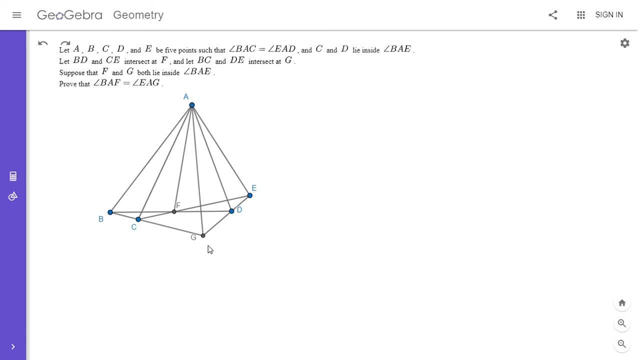 his proof. and what it does is it approaches it from a different angle. Instead of showing that angle BAF is equal to angle EAG, I'm going to let F prime be the point, so that BAF prime is equal to EAG, and then I'm going to show that E, F prime and C are collinear. 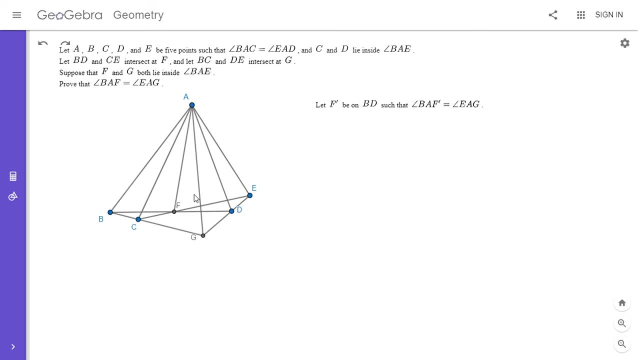 Okay, so let F prime be the point on BD, such that BAF prime is equal to angle EAG. Okay so we don't know that F prime yet lies on EC, and that's what we're trying to prove. and if we could do that it would solve the problem And the reason that we're approaching. 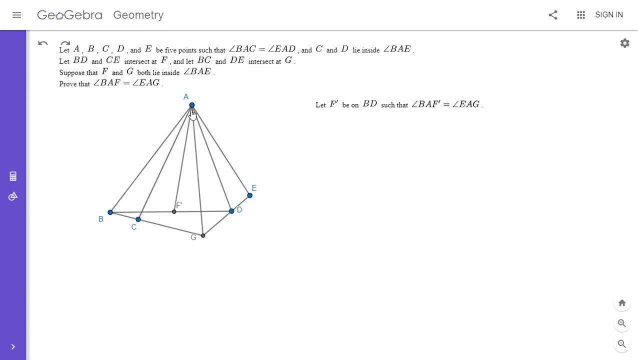 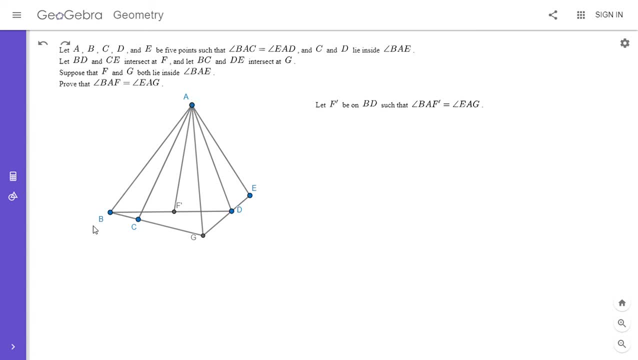 BAE, The lines AB and AE are symmetric with respect to that angle bisector, The lines AC and AD are symmetric with respect to it, And the lines AF, prime and AG are also symmetric with respect to it. So we're going to sort of take advantage of that symmetry here. 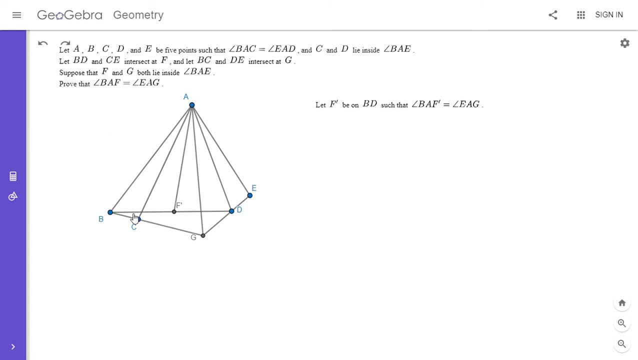 So I'm going to start by extending BG to meet AE at a point. So let BG meet AE at point H. And now what I'm going to do is so some of you who are familiar with cross ratios might know that the cross ratio is really a function of four lines. So if we look at the lines, 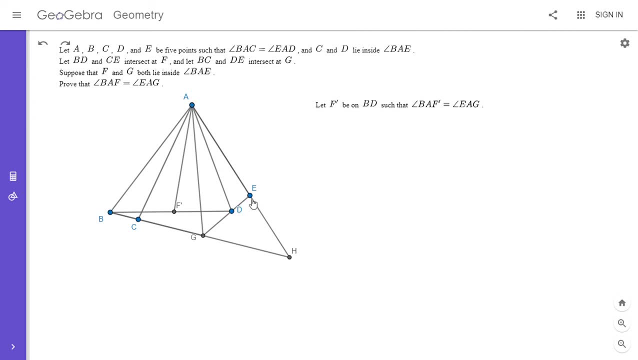 lines AB, AC, AG and AH. that pair of four lines has a cross ratio. So I've kind of on my channel, only spoken about the cross ratio of four points. but you can also think about it as being a cross ratio of those four lines, because if you take any other line and you intersect it in those four, 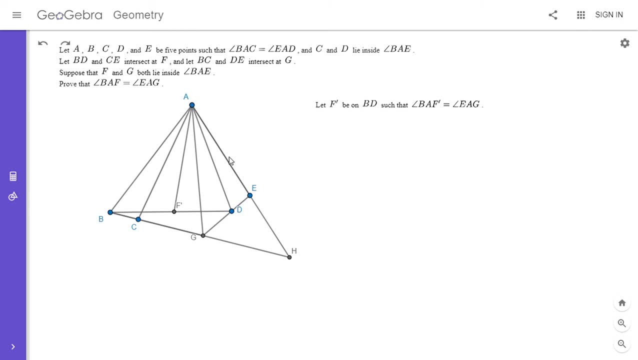 lines at four points, the cross ratio would have to be the same, So I'm going to use that here. So what I'm going to do is I'm going to reflect these four points- BC, G and H- across the angle. 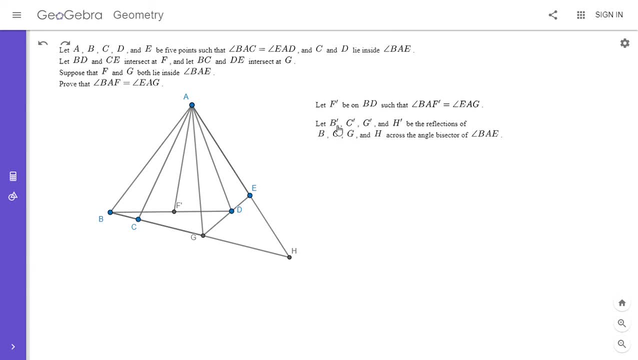 bisector of A, And I'm going to let them be B', C', G' and H' And those reflections of these four points across the angle bisector, using that symmetry, they're going to lie on the lines AE, AD, AF. 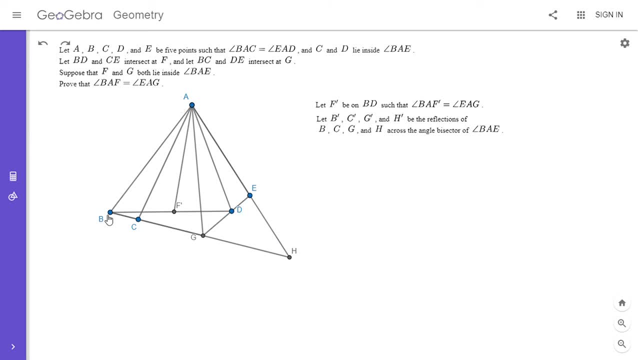 I think that should be right, So I am going to write this out. So B', C' G' and H' by symmetry would lie on the lines AE, AD, AF' and AB. That's because angle BAC is equal to angle EAD. 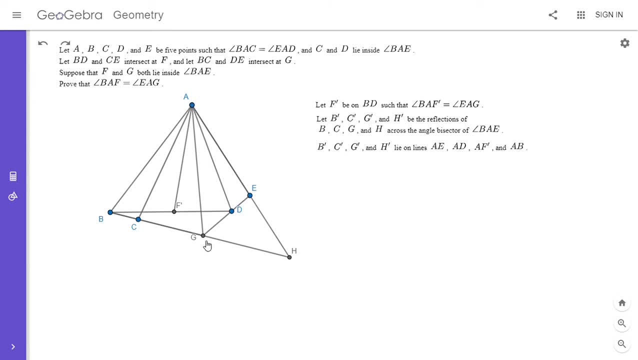 and angle BAF' is equal to angle EAG. So if we reflect across the angle bisector of BAE, we'd have to get that this is true. So I'm going to draw those four points: B', C', G' and H'. 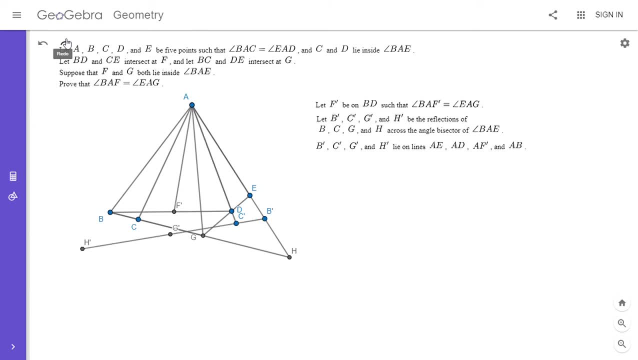 Okay, And they all have to lie on those lines that I mentioned: AE, AD, AF' and AB. All right, And now we can use symmetry here. So if you look at the four points, B, C, G and H- 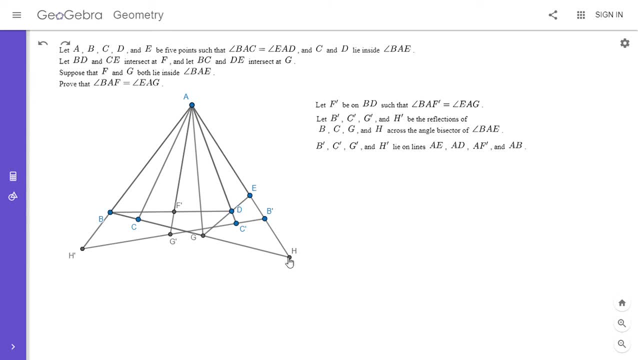 and you look at the distances between them, it has to be the same as the distances between B', C', G' and H'. Okay, Because by symmetry, all four points here are a reflection of all four points here, And so that means that the cross ratio of those four points has to be the same. 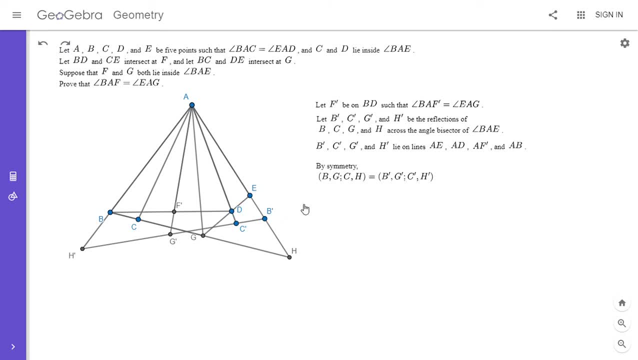 So I'm going to write this out. So, by symmetry, the cross ratio B, G, C, H has to be the same as the cross ratio B', G', C' H' Okay, And so that's the whole reason why I constructed those four. 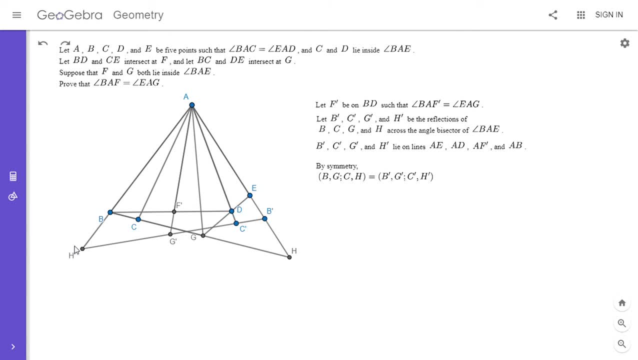 points. But now what I'm going to do is I'm going to try to project them through point A onto this line BD. So in order to do that, I'm going to extend BD to meet AH at a point. So I'm going to let it meet AH at a point F. 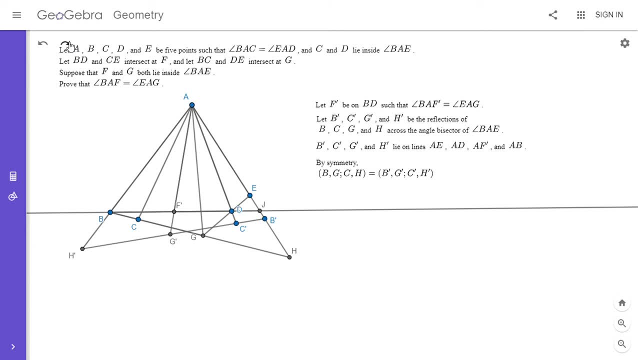 And- or actually I'm going to call it J- And if you project these four points through A onto line BJ, you get another cross ratio. So B would go to point J, G' would go to point F', C' would go to point B and H' would go to point B. Okay, So now that we have this cross ratio is 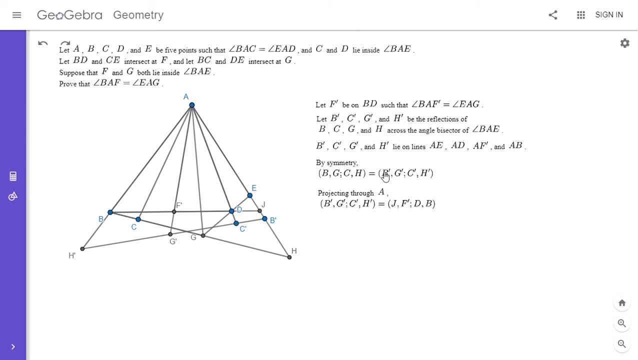 equal to this cross ratio. I'm going to go ahead and project these four points through A onto line B. I'm going to erase points B', G', C' and H' because the whole reason that I constructed them was to prove that this cross ratio would equal this cross ratio. Okay, so I just erase them, All right. So 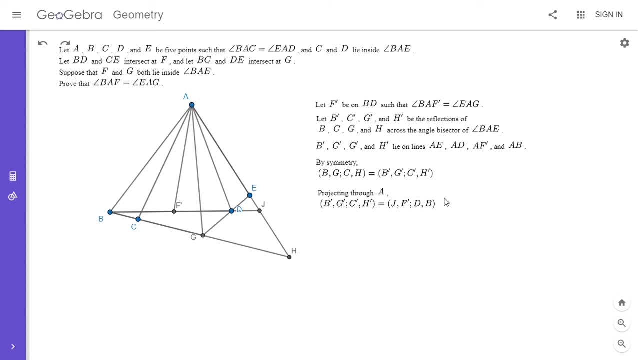 now there's a certain trick with cross ratios where if you have one cross ratio and you swap the two letters outside the semicolon, you're going to have a cross ratio that's equal to this cross ratio, And then you swap the pairs within the semicolons, it's still the same thing. So this cross ratio. 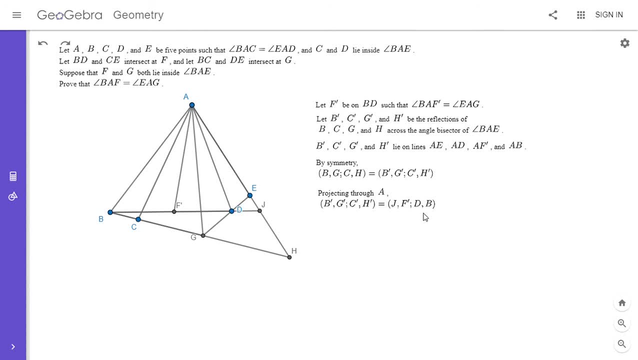 should be equal to B' J. So I'm going to actually show a short proof of that here, but it's a good fact to just memorize, So here's the proof of that fact. So first I'm going to write out the definition of this cross ratio. Okay, So J'. 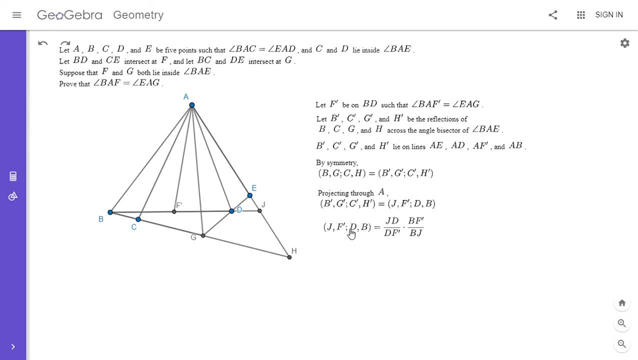 D' D' B' You look at what is the ratio. D divides segment J' F' into, that's J' D' over D' F' and then you multiply it by the flip of the other ratio. So you multiply it by B' F' over. 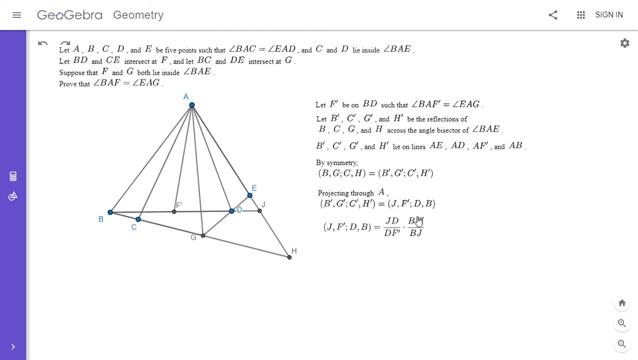 B' J. Okay, And now we can rewrite this. We can move B' F' to this fraction and J' D' to the other fraction. So algebraically this is the same as B' F' over D' F' times J' D'. 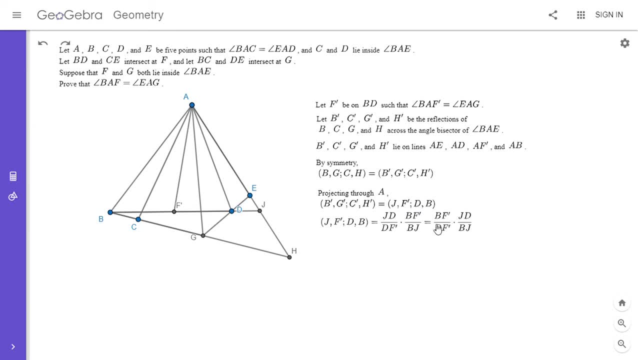 over B' J' And now we can look at this expression And it's easy to see that that is equal to the cross ratio B' D' F' J' Because this is the ratio that F' divides B' D' into And 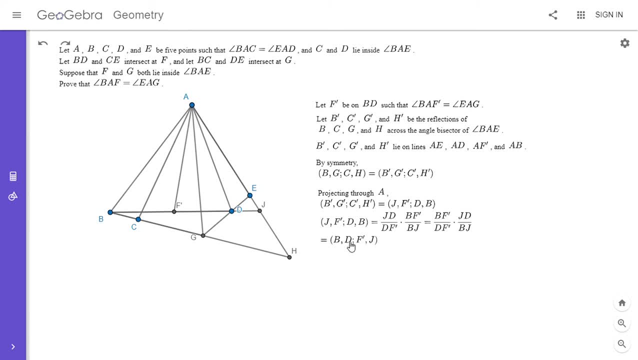 this is the reciprocal of the ratio J' divides B' D' into. So I just memorized this fact that this is equal to this. but here's the algebraic proof, right here. Okay, And the reason why I did that is because now I want to project through point E And you'll see. 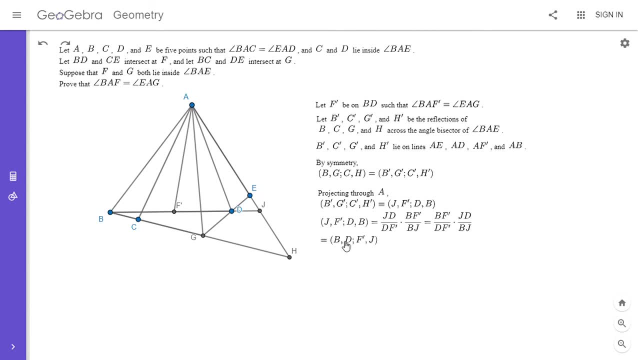 why this transformation is useful. Okay, So I'm going to take these four points- B', D', F' and J' and I'm going to project them through E' back onto the line B' H', So B' stays at B' D' E' would go to point G' F'- we're not sure yet where it goes- And J' 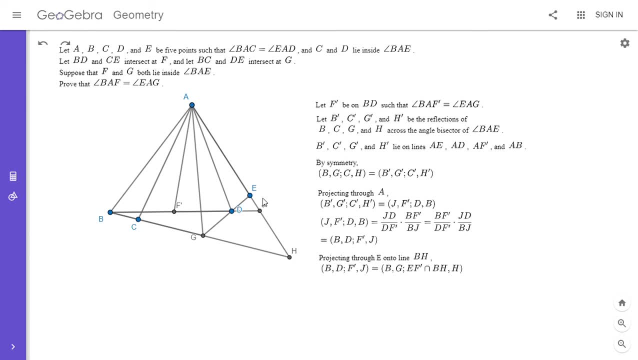 goes to H'. Okay, So this cross ratio B' D', F' J' is equal to B' G' because point D' goes to point G' And then F' I don't know yet where that goes, So I'm just going. 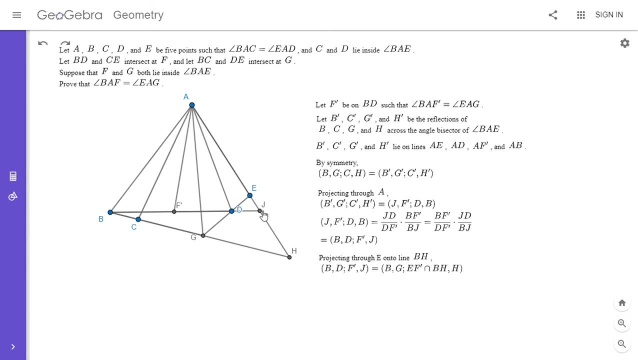 to put E', F', intersect B', H' And then point J' goes to point H'. All right, So we've almost solved the problem here, So we can use transitivity. So this original cross ratio has to equal this, which has to equal this, which is equal to this cross ratio.